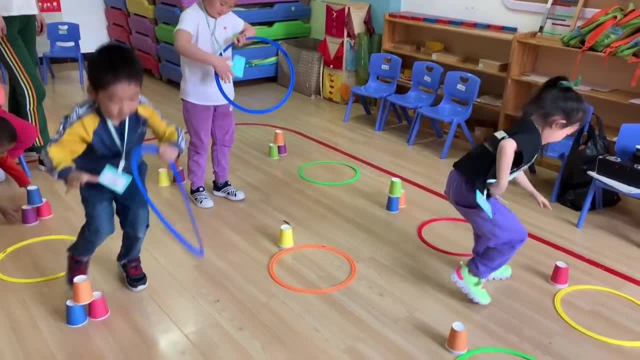 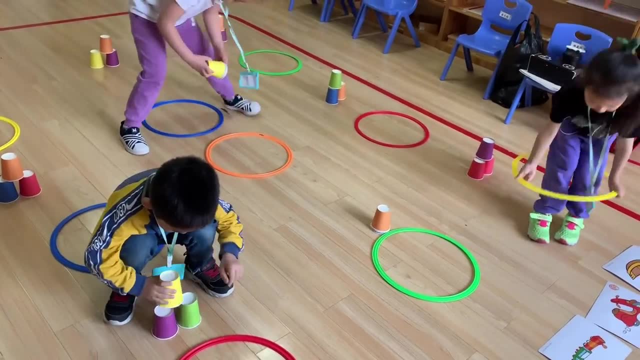 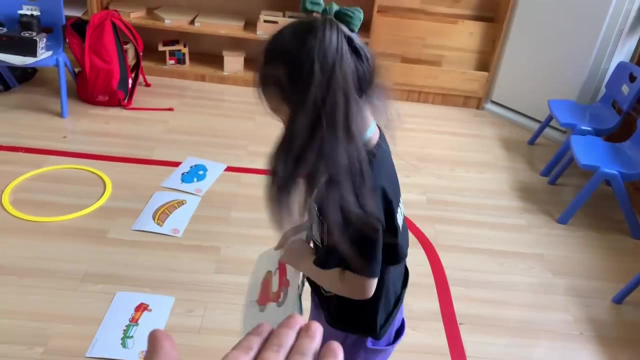 So to play this game, guys, all you have to do is prepare the cups and the rings or hula hoops alternately and put the flash cards in front of them. You can make two or three or four lines or columns of these paper cups and rings, depending on your space you've got, and the students you've got. 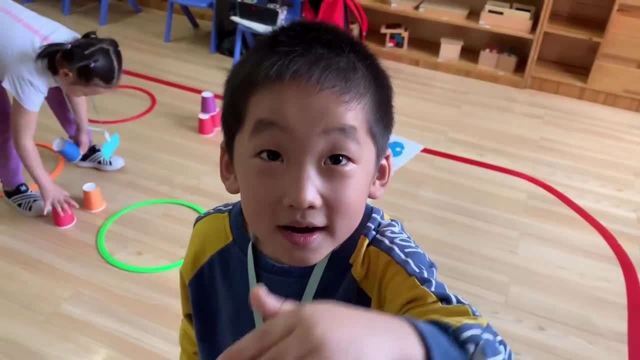 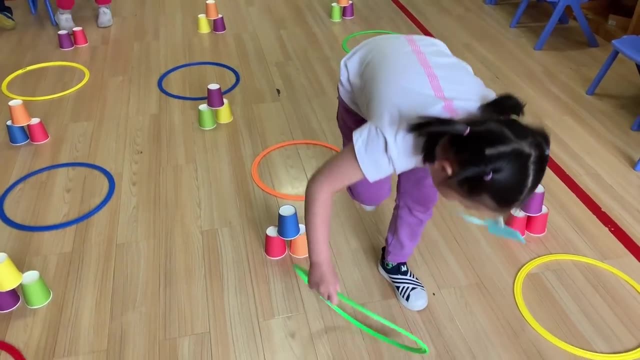 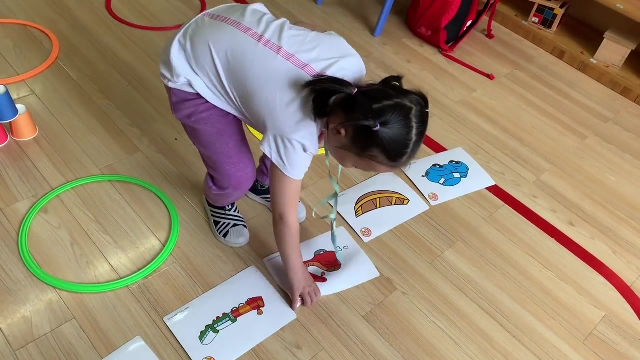 and the time you've got as well. So the aim of the players is to race to the flash cards by forming the three cups into a pyramid and then pick up the rings or hula hoops, and they have to go through it from head to toe until they reach the flash cards and practice the 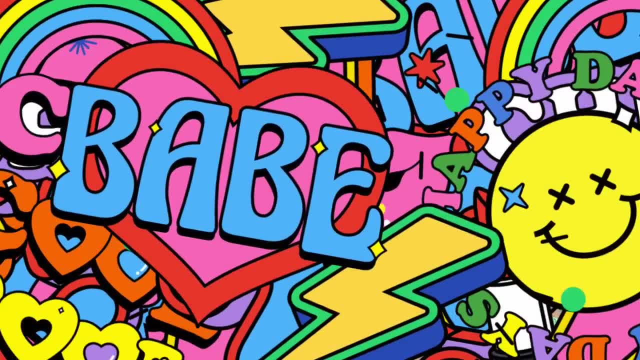 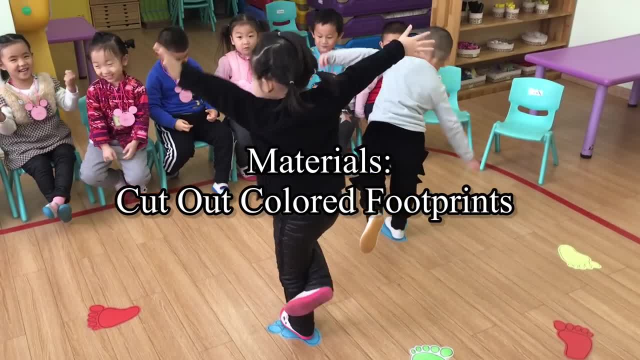 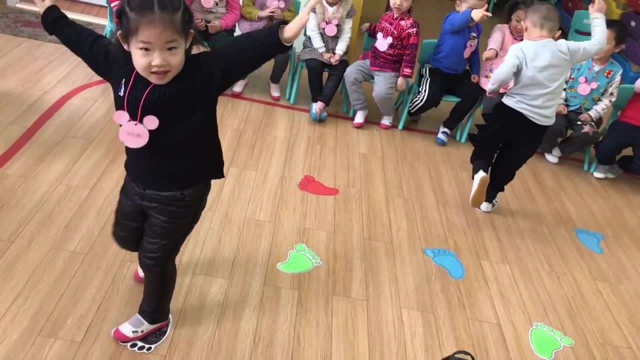 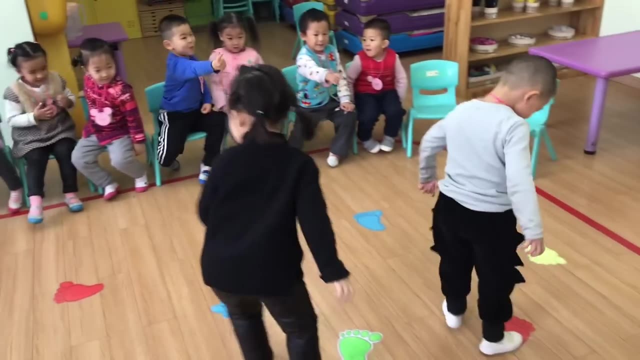 word. It's like a relay game, Game 3.. Hop-on Materials: Count out colored footprints. So, guys, to play this game, you need to prepare, cut out colored footprints beforehand. In this situation, my lesson is about colors, so I have some footprints on colored papers and then I laminated them and cut them out. 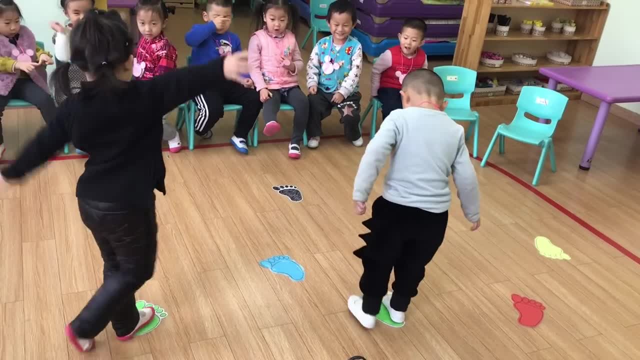 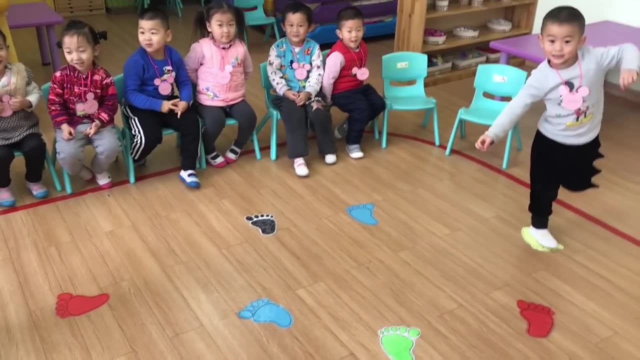 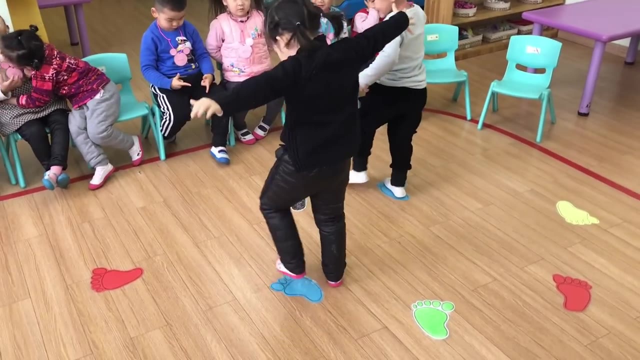 Once you're in the classroom, all you have to do is spread out these colored footprints and then you can call out two students and the teacher will have to say a color and then the students will have to search for it and then hop on it and say the word or practice the target words. 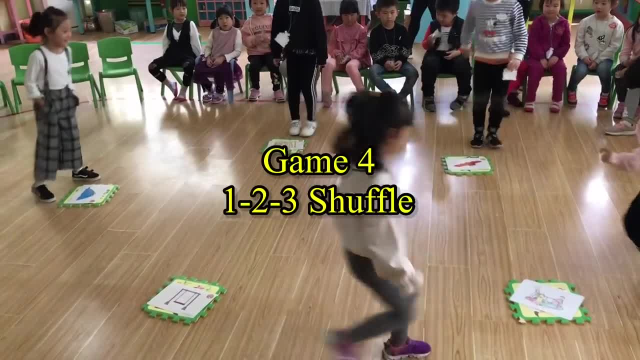 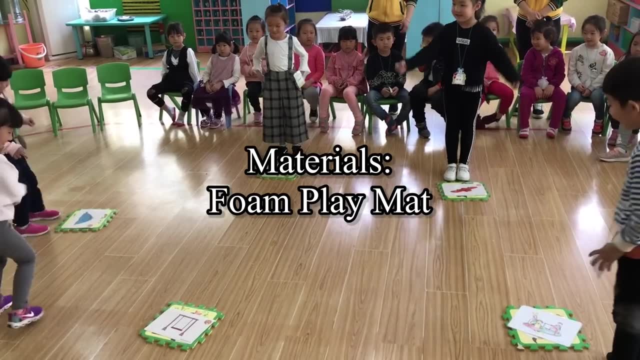 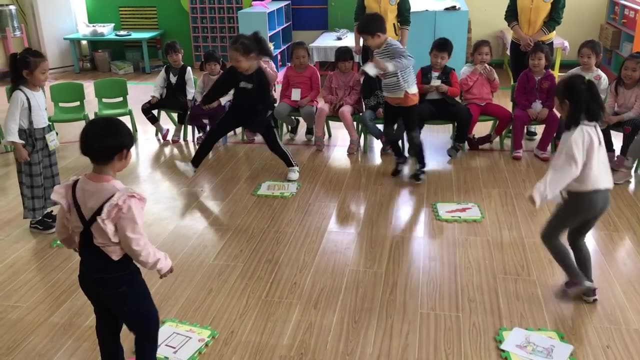 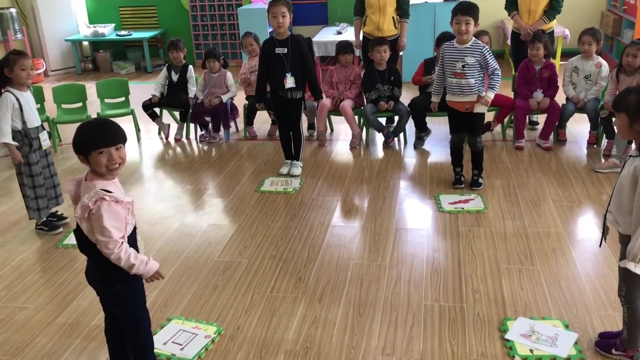 Game 4.bck. game 4: 123 shuffle. was this just an usual granny dance? So to play this game, guys, it's pretty easy. All you have to do is take some foam clay mats in the classroom. You can arrange four or five or six foam clay mats And arrange them in a circular setting. 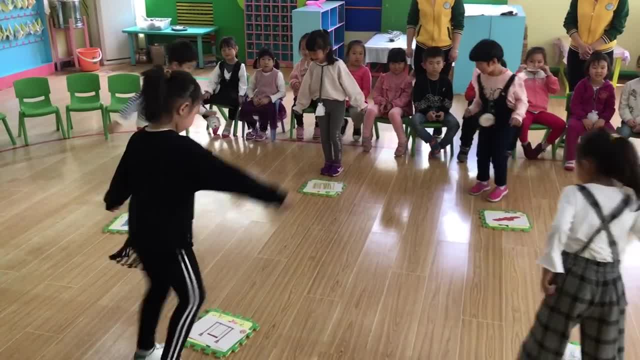 or not, maybe something else, But they don't look so satirically right, xD? or not, Its alright. Yeah, But you can hit the 100 leaf Ponthats with your hands and you can use those flash cards on them and then call out the students and they have to stand in. 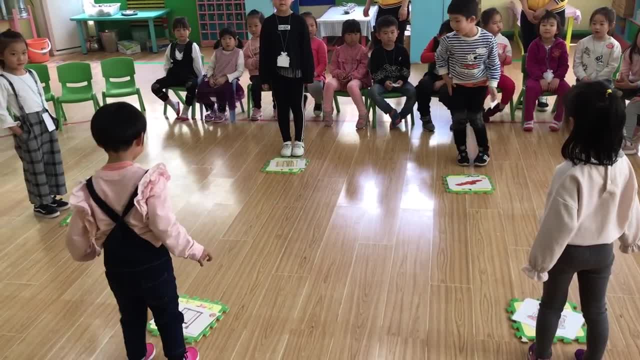 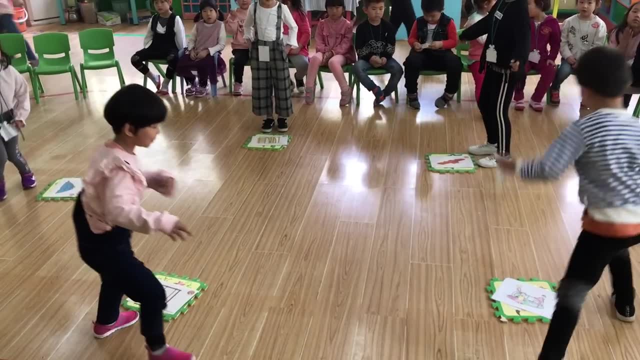 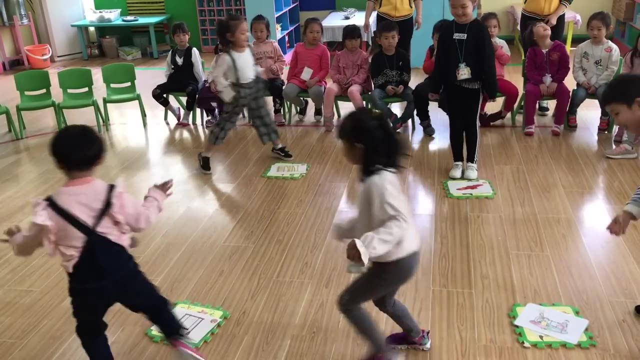 front of these floor mats or foam play mats, and when you say one, they have to go to their right, and when you say two, they have to go to their left. you know, you can play around with numbers one and two until until then, when you have to. 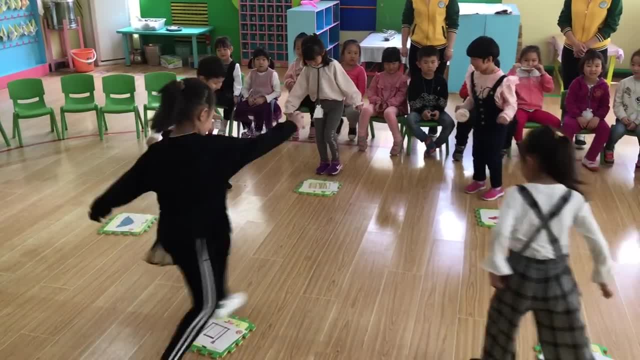 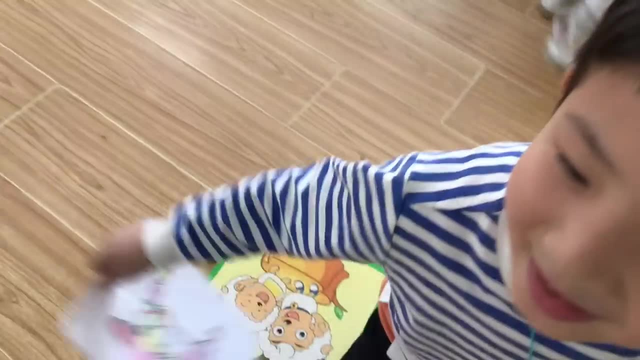 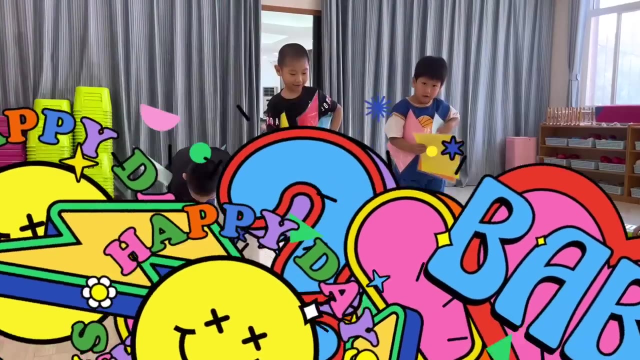 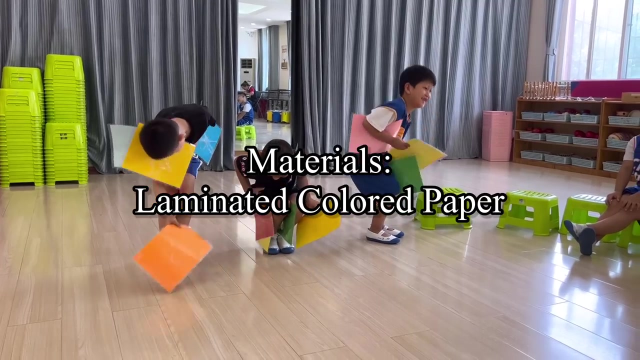 say number three. they have to shuffle or exchange places and then they have to identify or practice the target word which is on their designated foam. play mat game. five Japanese walk race materials: laminated colors or paper. so, guys, the mechanics of this game is kind of challenging. in the 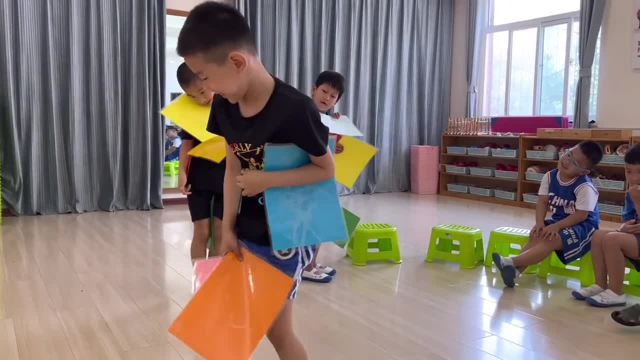 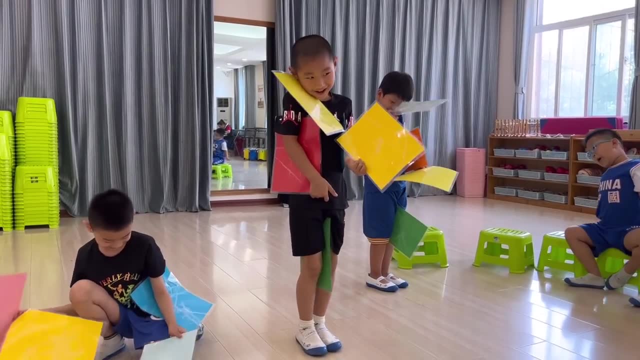 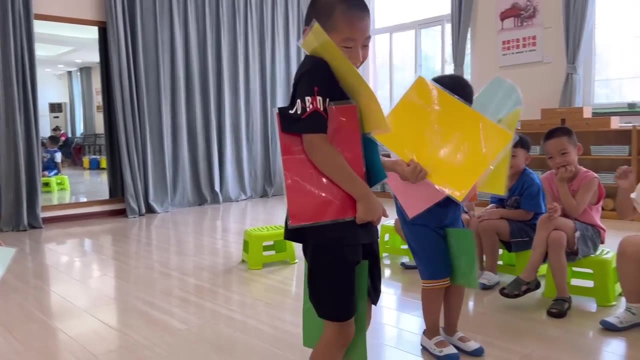 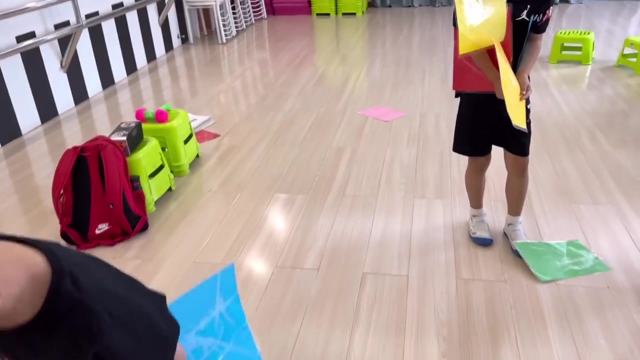 beginning, but once they've got it it's very interesting and fun to play with. so this game mimics the Japanese girl who wears the traditional dress, and they have to walk like you know, like a Japanese girl, by putting these four or five colored between their knees, between their armpits and between their neck and 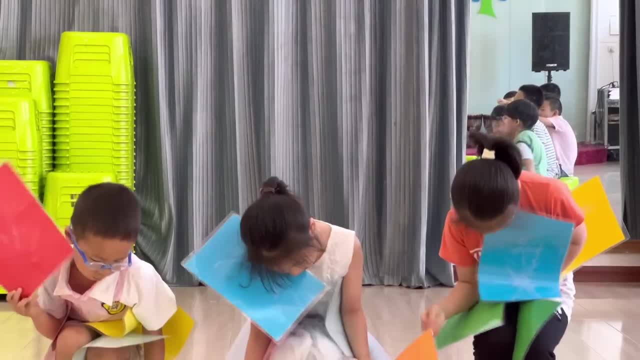 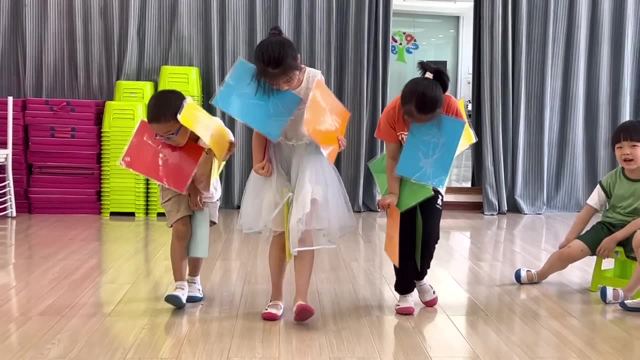 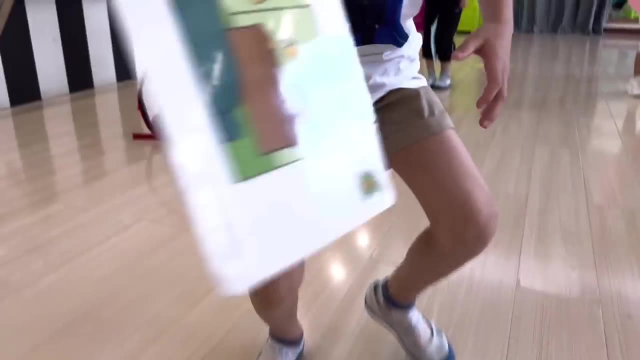 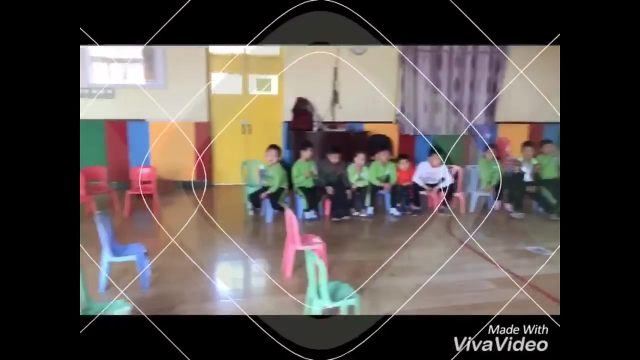 shoulders and then they have to get one of the papers which will act as their fan. so they have to walk like a Japanese towards the flashcards and once they've reached the flashcard they have to say the target words. I mean: gain six. inflatable balloon sticks. race materials- inflatable balloon. 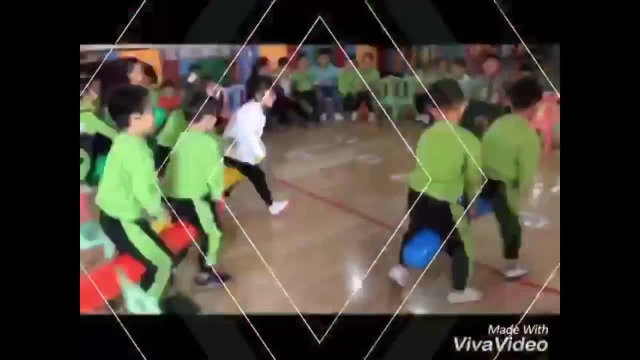 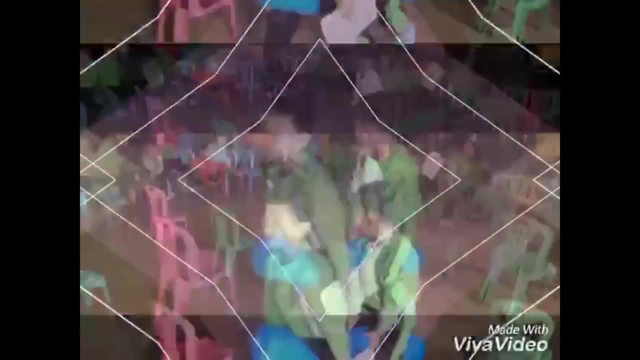 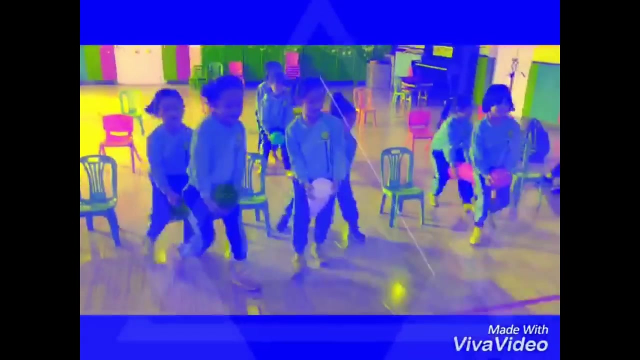 sticks and chairs. so, guys, to play this game you need to buy inflatable balloon sticks beforehand, and you know you have to inflate it before the game starts and then arrange the chairs into several columns. it depends on how you arrange it. it will stay on the same size for all the time and it's very hard to find a. 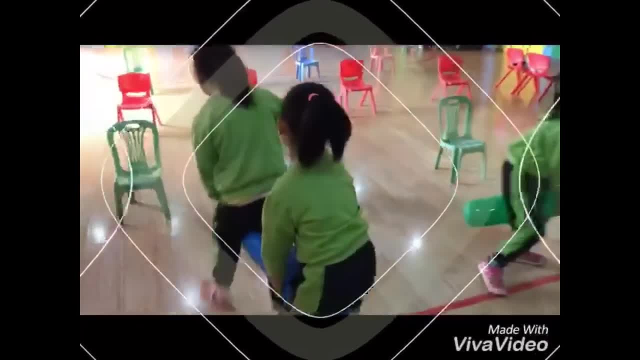 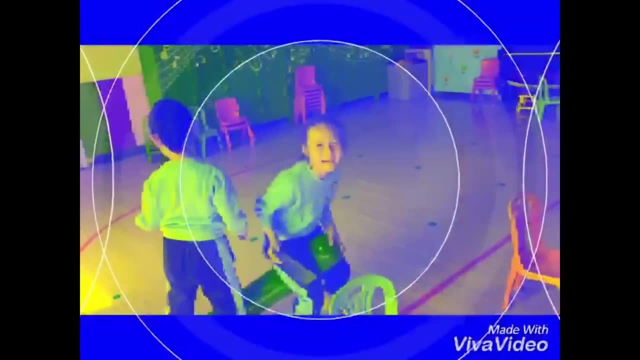 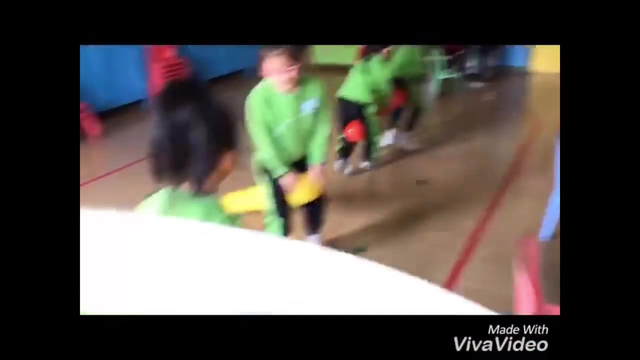 serve as their you know um trail or guide. they can go in a zigzag motion, just like what you see in the video, or they can just go through the lines, uh, you know uh- directly to the flash cards in front of them. so you can play this game, uh, by twos or by pairs, and they have to ride on the inflatable. 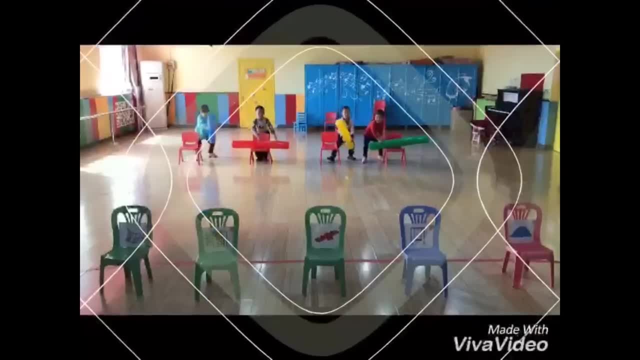 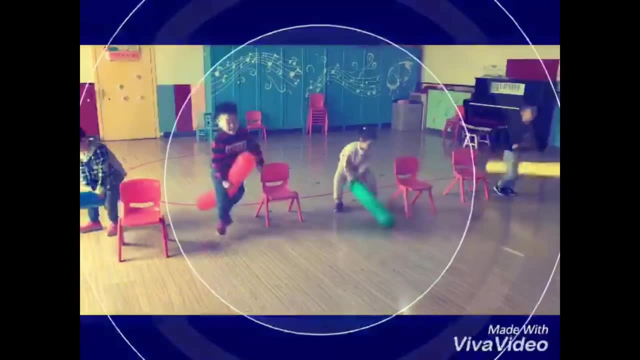 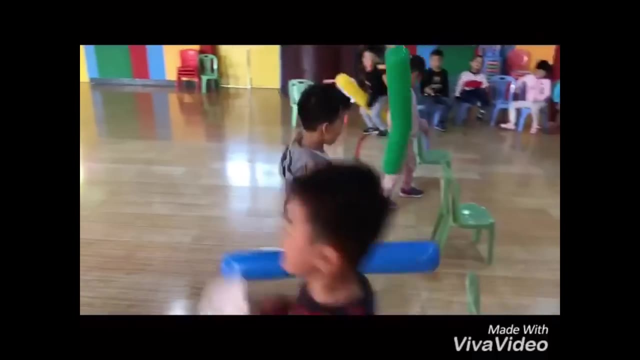 balloon sticks. the second option is you can play this game individually and then ask the students to put this inflatable balloon sticks between their legs or between their knees and they have to jump off to the flash cards and back to their chairs and say or practice the target words. 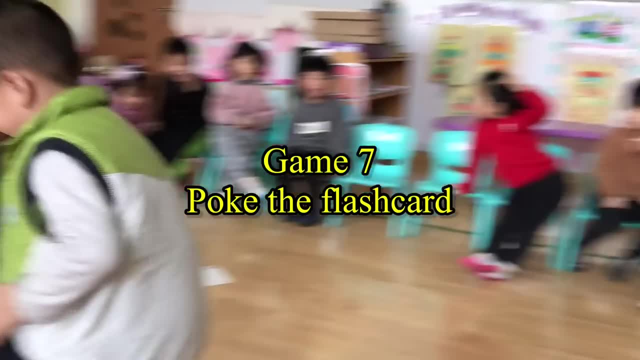 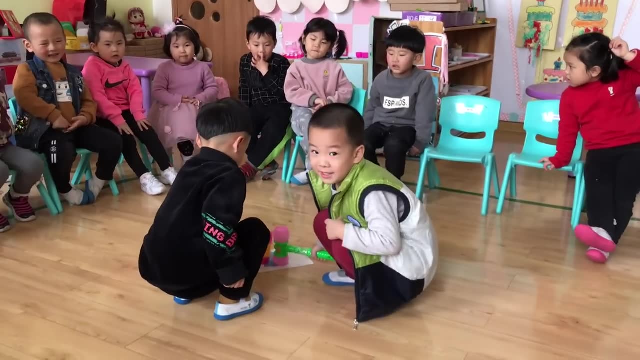 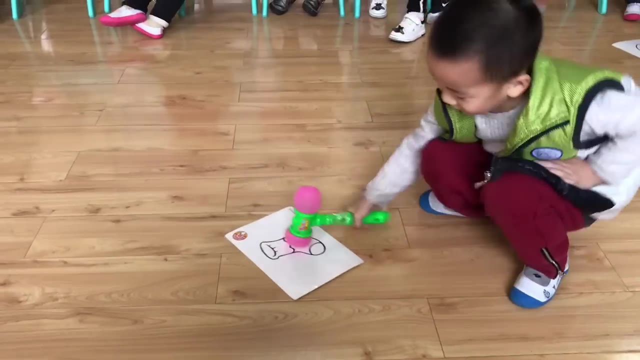 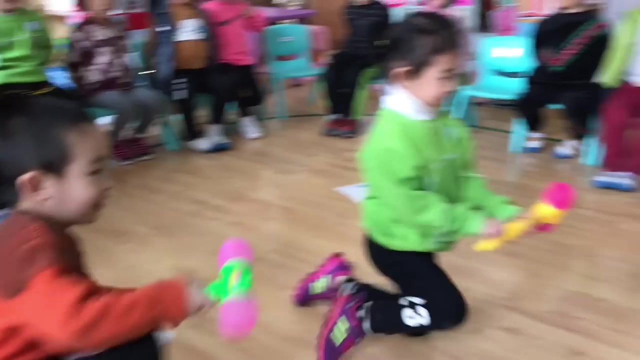 game seven: poke the flash card, materials, materials, materials. so, guys, this is probably the simplest and easiest game that you can do in your classroom. all you have to do is, you know, take two or three or four- uh, toy hammers in the class and then you have to. 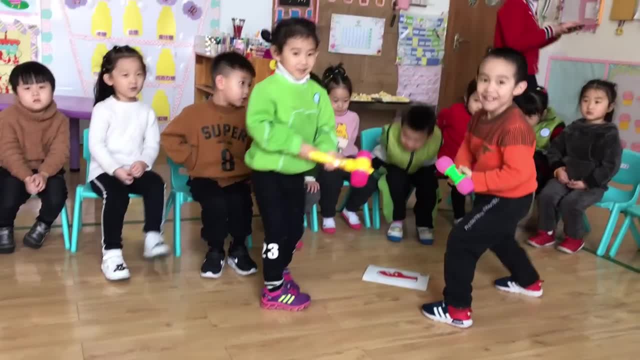 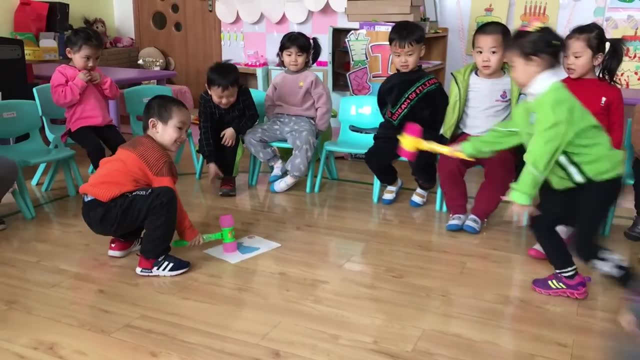 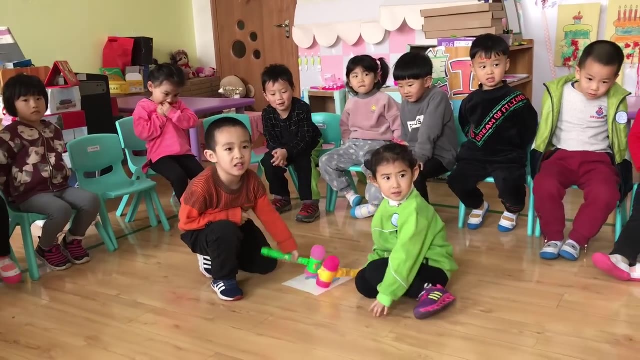 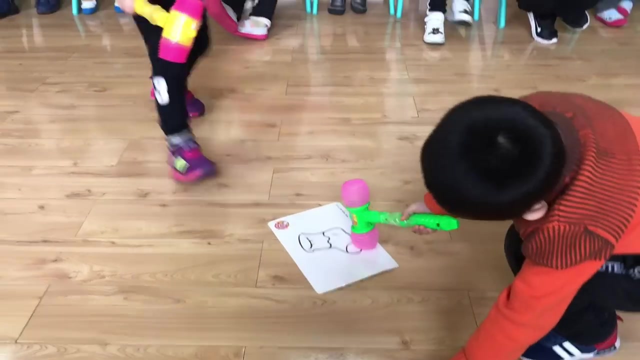 scatter the flash cards around the classroom in front of the students, and then you can call out two or three students- uh, depending on the, depending on your liking- and give them or hand them out those um toy hammers, and then the teacher will say a word and they have to search for that flash card and then poke it and say or blurt out: 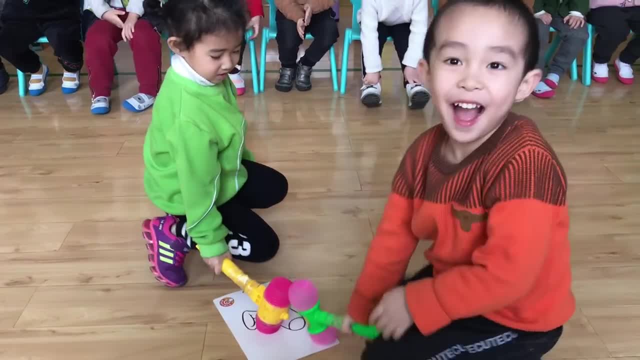 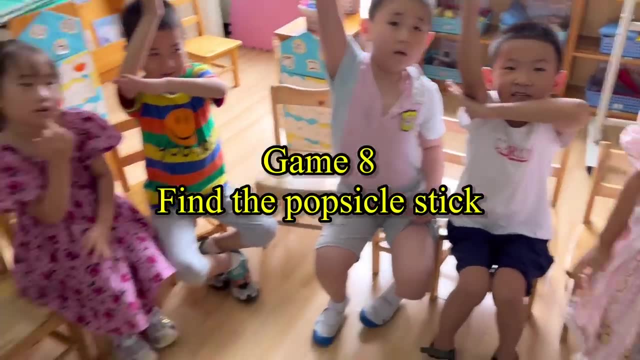 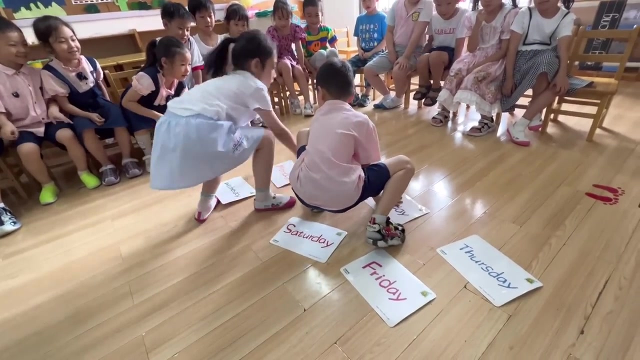 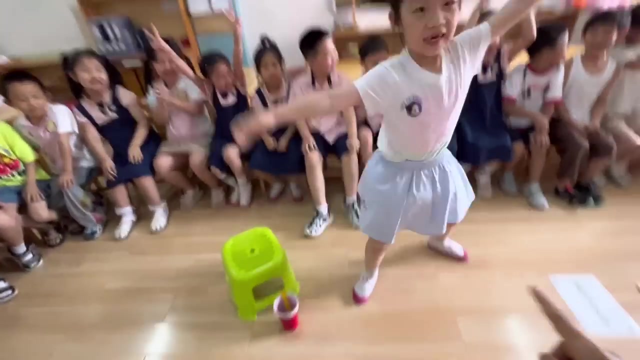 the target words loudly in front of the class. find the popsicle stick materials, popsicle sticks. So, guys, the mechanics of this game is quite simple. All you have to do is spread out the flashcards on the floor, And opposite to those flashcards are two chairs. 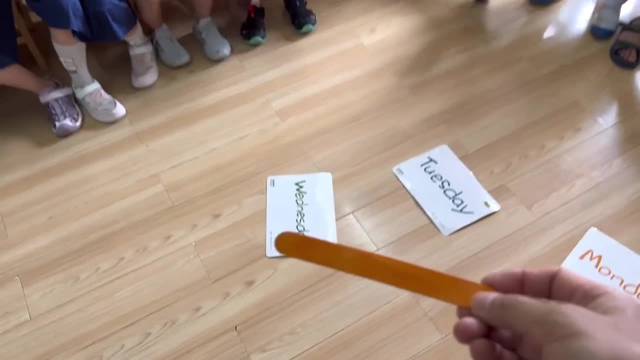 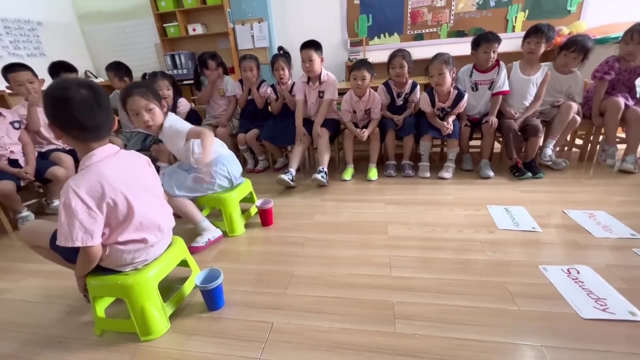 Call out two students to sit on a chair, Hide a Popsicle stick under one of those flashcards, Then give a go signal And then the students will have to find or search for a Popsicle stick. The first one who found a Popsicle stick gets a point.